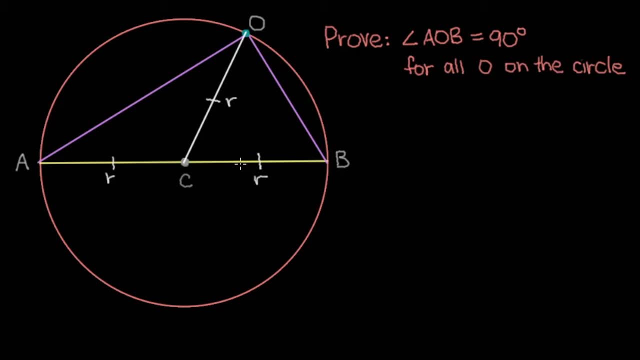 the principle of isosceles triangles, that says the angle opposite of the equal sides must be equal as well. So if we call the angle opposite of CO in the triangle BCO x, then the angle opposite of CB must be x as well. By the same reasoning, if the angle opposite of CO in the triangle ACO is y, 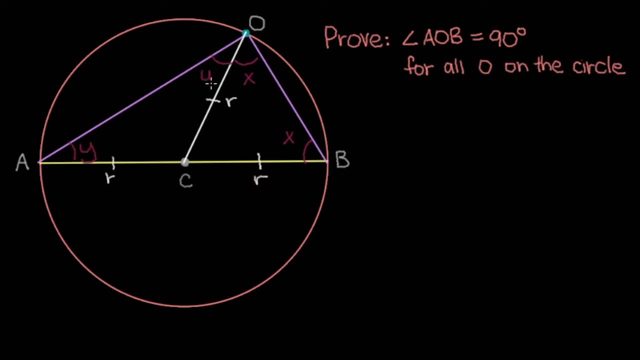 then the angle opposite of AC must be y as well, And you'll notice that x plus y is equal to our angle AOB, And we're trying to prove that this thing is 90 degrees, Because the sum of the angles in a triangle must be equal to 180 degrees. we know that this angle must be 180 minus 280. 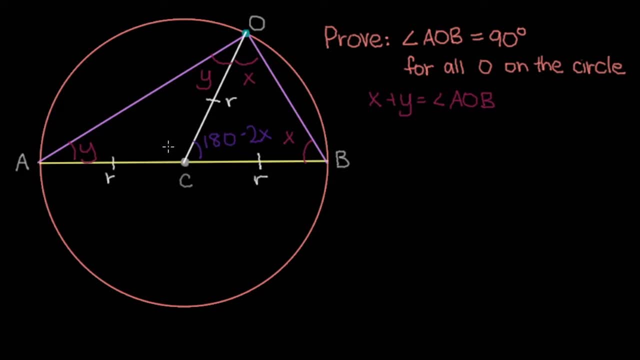 And the same thing applies for triangle ACO. This angle over here must be 180 minus 2y for the angles in this triangle, to sum up to 180 degrees. Now we must notice the angle ACB is equal to 180 degrees because the angle ECB is the 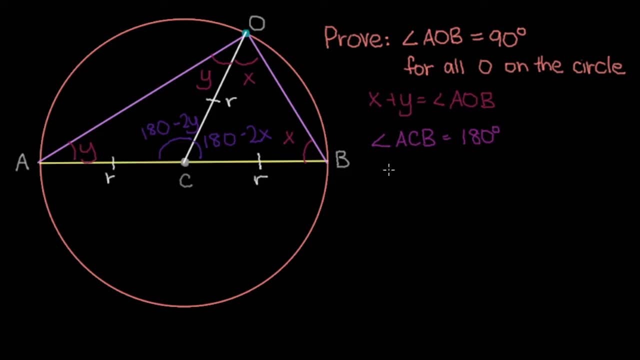 angle of a straight line. Now, the angle ACB is composed of two parts. It's the part on the left, which is 180 minus 2y, plus the part on the right, which is 180 minus 2x, and this must equal 180 degrees. 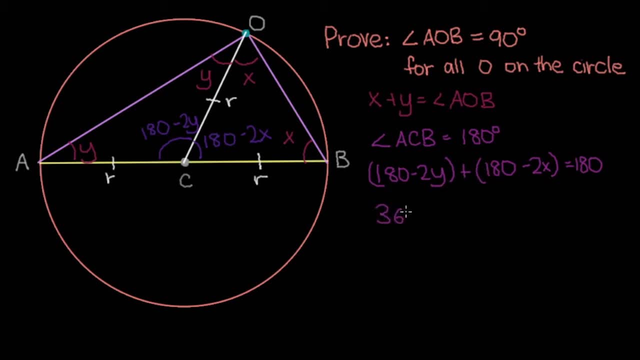 Now, if we add these two terms together, we get 360 minus 2x. minus 2y equals 180.. Subtracting by 180 on both sides gives us 180.. So if we add 2x and 2y to both sides, we get 180 equals 2x plus 2y. and dividing by 2 on 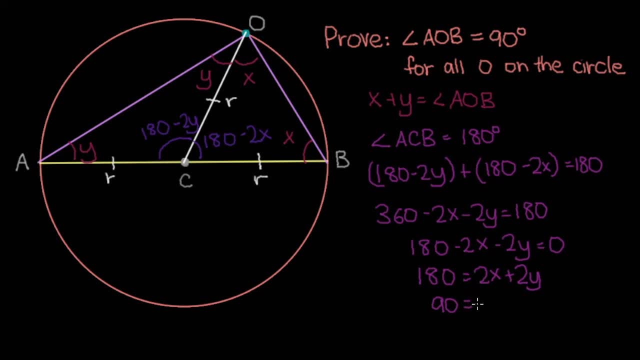 both sides gives us 90 equals x plus y. Now we should remember that x plus y is equal to our angle, AOB. And if x plus y equals 90 degrees, then AOB must be 90 as well. And thus we have proved that if we are given a circle with diameter AB and we choose any, 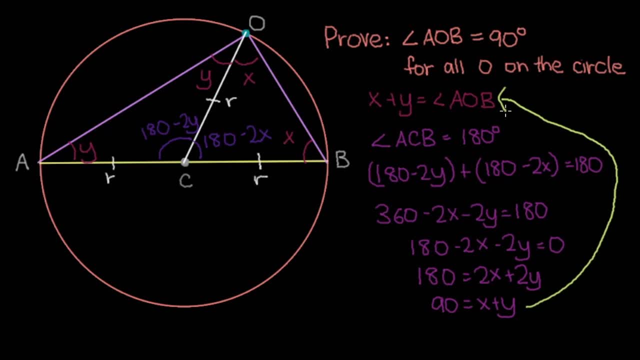 point O on that circle, then the angle AOB is 90 degrees.